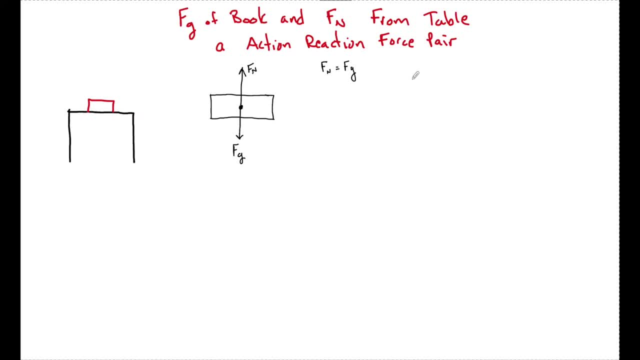 FG, but that does not mean that they are an action-reaction pair. In fact, these two forces are not action-reaction force pairs, And there's going to be two ways that I can really explain this to you. The first is very simple, by looking at the definition of Newton's. third, I have a 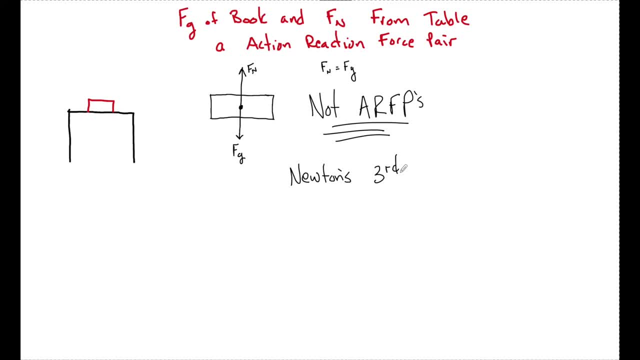 really in-depth video about Newton's third. that's going to go into it. But in that video I talk about how I hate the definition of every action has an opposite and equal reaction. You can watch that video if you want to see really why I hate the wording of that. So I tend to not 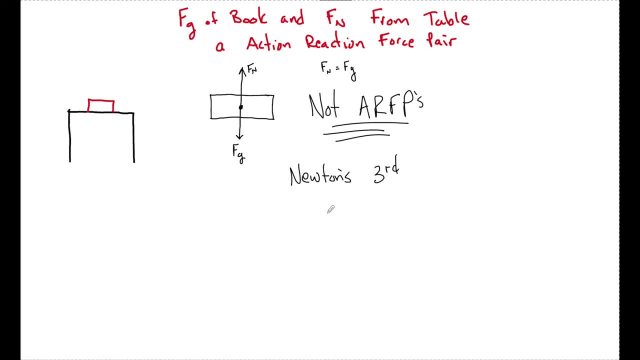 use the words. when I list Newton's third law, I say that there is a force vector of one object on a second object that must be equal to the opposite force vector of two onto one. There's something that needs to be seen here, which is going to prove that this is not an action-reaction. 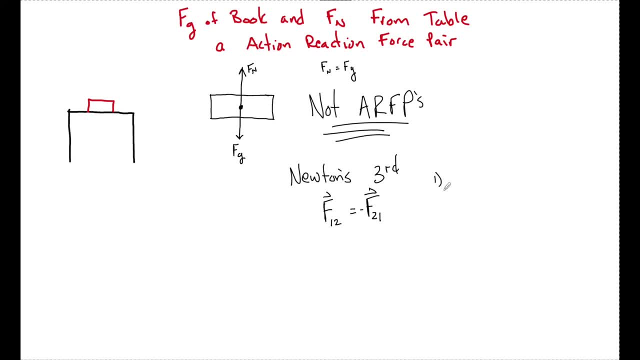 pair. First and foremost, for Newton's third law to apply, you need two objects. right, We need object one applying a force onto object two. In this case, the force of the normal is acting on the book And the force due to gravity is also acting on the book, So there is only one object. 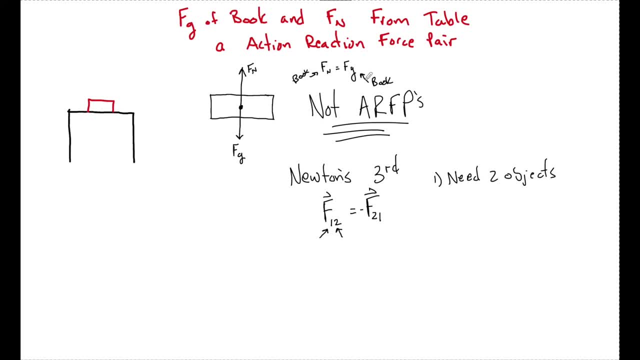 These are not action-reaction pairs, because these two forces act on only one object, And, guys, that might make things a little bit more confusing than they need to be, But what you need to understand is that an action-reaction force pair first and foremost needs to have two objects. Now 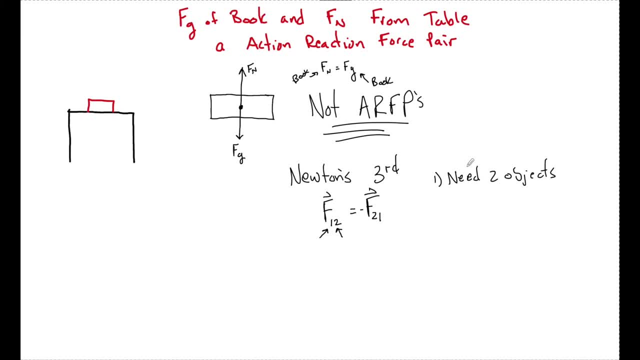 generally, when we have an action-reaction pair, they're both going to be the same exact type of force. They'll both be a pull, They'll both be a push. They'll both be from gravity. okay, This is a reaction to the book hitting the table. It's not technically a reaction to gravity, It is a result. 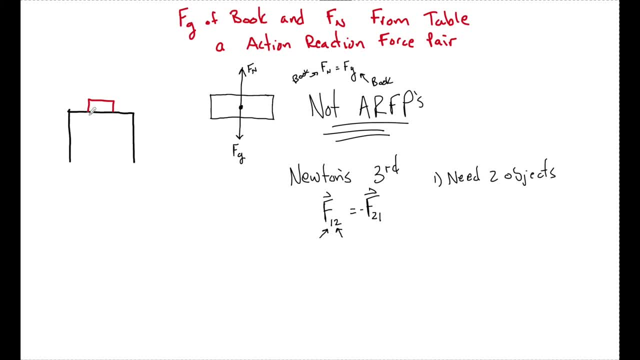 of gravity coming down and actually deforming the table a little bit, And then the force of the normal is really restoring force. Like I said, I don't want to get ahead of myself too much, but there are two forces that act on the book: gravity and the force of the normal. There are actually 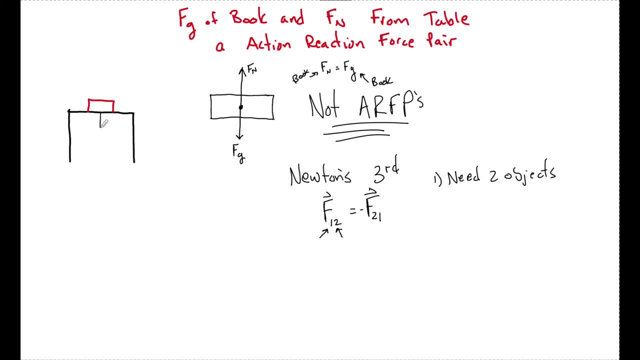 three forces that act on the table. We have the weight of the table, Fg, We have the normal force, Fn, but also we have a force that the book applies F12 onto the book. And then there is a force 21 that acts And those two are an action-reaction pair but they are not equal to Fg And, like I, 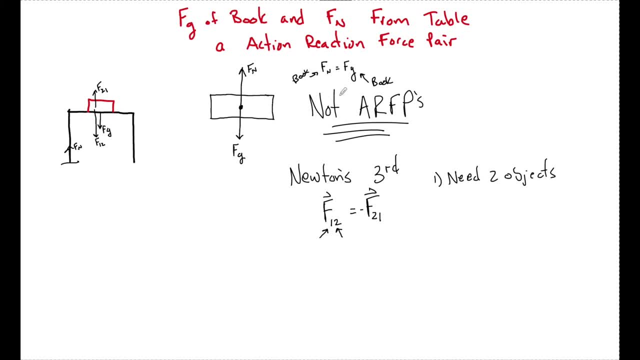 said. that's way more than in depth than I really need to go, But the simple answer: Fn and Fg are not an action-reaction pair because they act on only Fg One object, where an action-reaction pair needs two objects, a pair of object, object one and object. 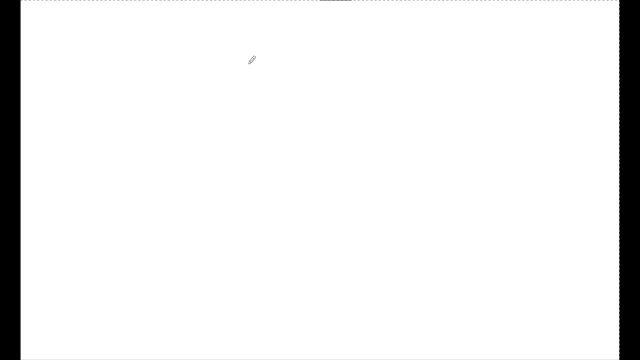 two. And the next misconception I want to talk about is, like I said, if there's an action-reaction force pair and they're equal and opposite, shouldn't we not be able to move? And the real reason behind that is: we can't forget about all of Newton's other laws And it really has to deal. 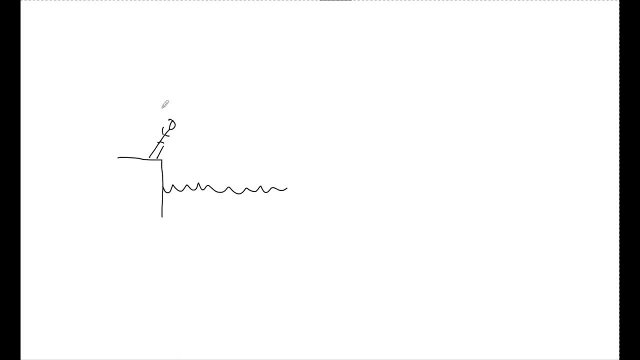 with mass. And here's what I mean. Here's me: I, I say, have a mass of 60. I have a mass of 60. I have a mass of 60 kilograms. Okay, Now, this is the dock, and the dock has say a mass of a thousand. 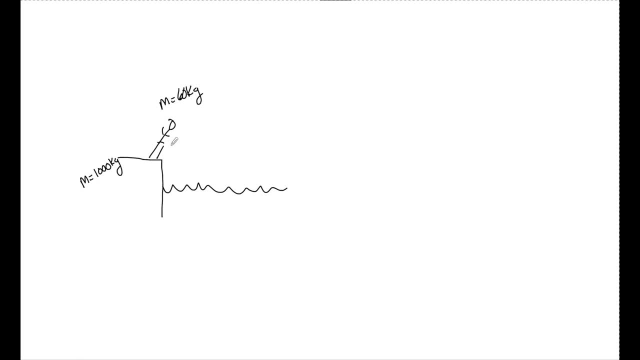 kilograms. Okay, Now, what allows me to jump from here to here? Well, yes, friction, but let's not get too in depth. What we are going to see is that, me, I am going to push on this deck. That is my. 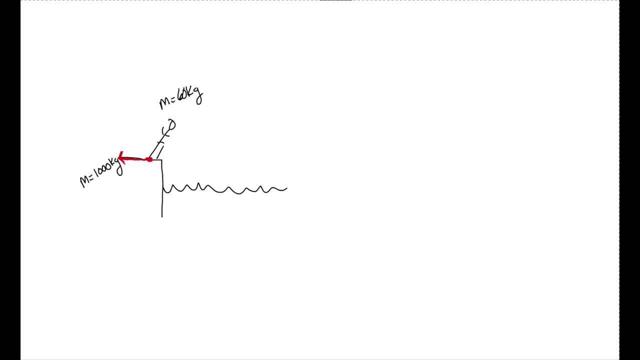 action force. Now, Newton's third law says that because I push on the deck, the deck is going to then push on me with an equal and opposite reaction force. But if we gave that force a number, let's say that force happened to be one. Newton of force. 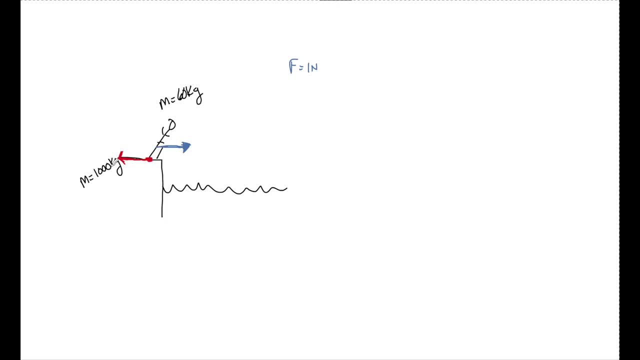 Well, we'd see that I'm not able to really accelerate this deck. If we look at Newton's second law and if I apply a one Newton force to a 1000 kilogram object, the acceleration of that object is going to be next to nothing. Where, if I take the Newton's